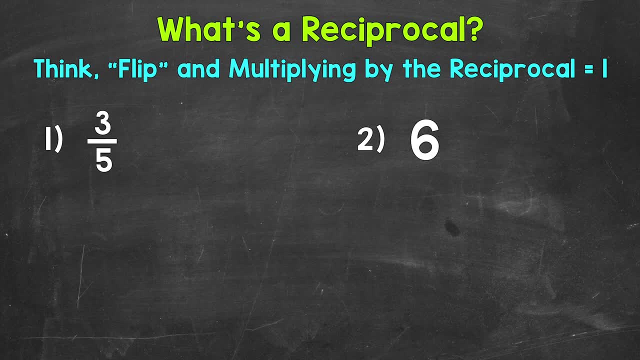 Reciprocals are used throughout different areas of math, For example when dividing fractions or certain algebra problems, So it's a good idea to be familiar with reciprocals. Let's jump into our examples, starting with number 1, where we have 3 fifths. 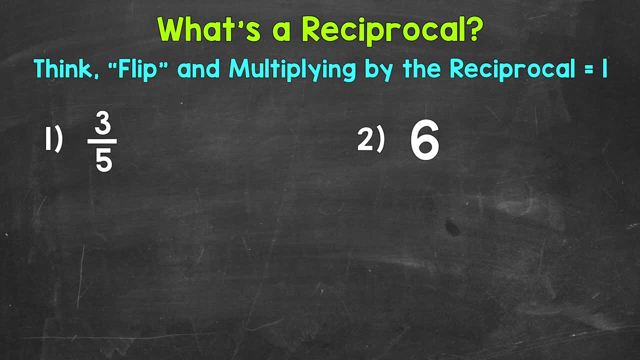 So let's find the reciprocal, and we do this by flipping the fraction. So the denominator the 5, is going to become the numerator And the numerator the 3, is going to become the denominator. So we are flipping the fraction. 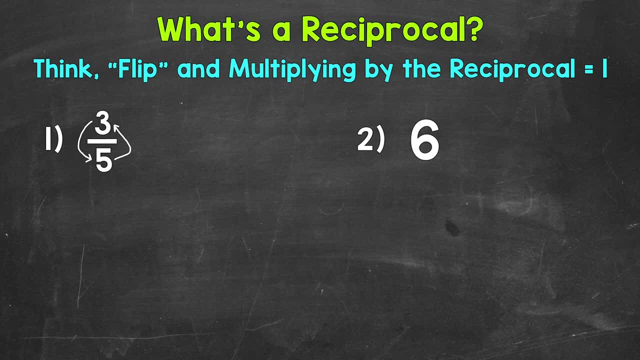 The reciprocal of 3 fifths is 5. 5 thirds. So that's our reciprocal. Now let's multiply our fraction 3 fifths by the reciprocal 5 thirds to show that we get 1 when we multiply by a reciprocal. 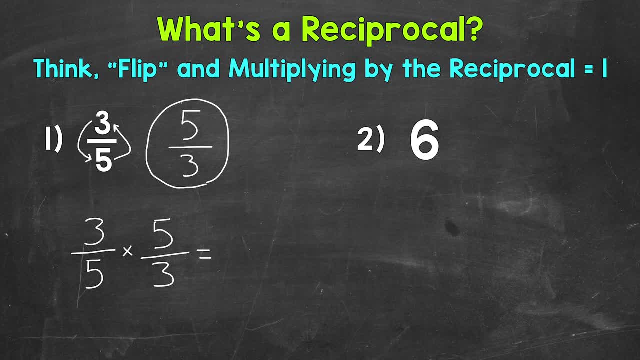 So let's multiply straight across. The numerators 3 times 5, 15.. The denominators 5 times 3.. So we get 15 over 15, which we know is 1.. Whenever you have the same numerator and denominator, that fraction equals 1.. 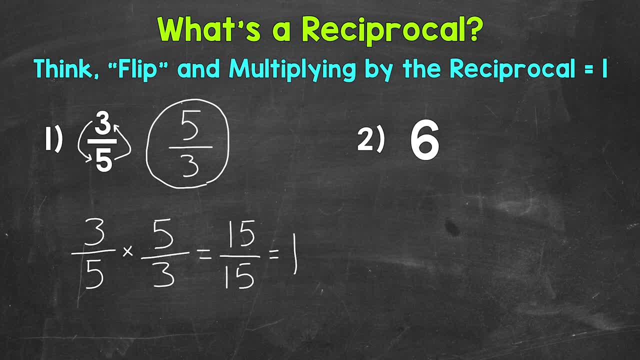 Let's move on to number 2, where we have 6.. For this one we have a whole number, So the first thing that we need to do is write this whole number in fractional form. That way we have a numerator and a denominator and we're able to flip that fraction. 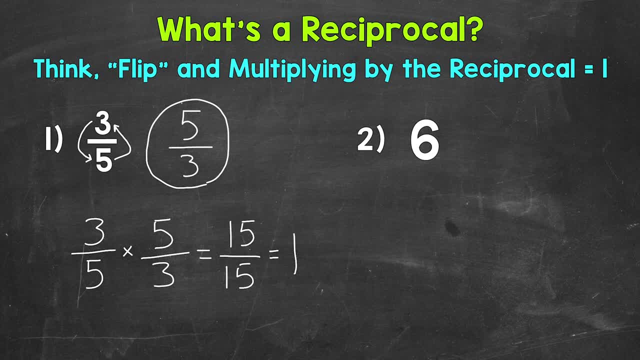 So to write a whole number in fractional form, all we need to do. I'll rewrite it underneath here. we put that whole number over 1. So that's 6 in fractional form. Now we're able to flip. So our denominator becomes our numerator and our numerator becomes our denominator. 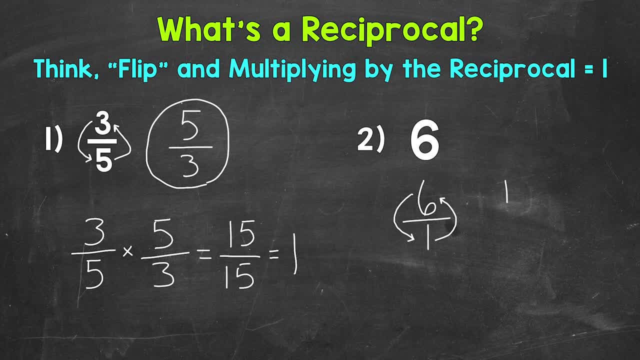 So the reciprocal of 6 is 1 sixth. This is our reciprocal. So let's multiply our whole number in fractional form, 6 over 1, times 1, sixth, to show that we get 1.. So numerators, 6 times 1 is 6.. 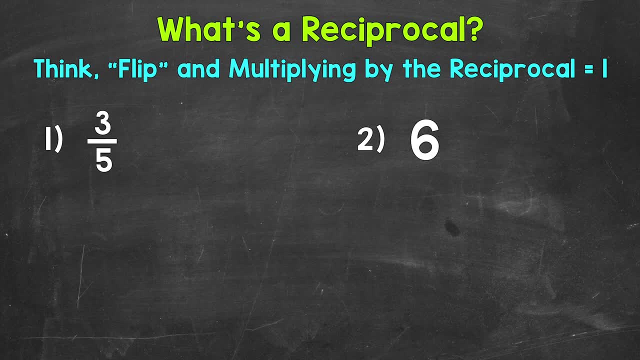 Reciprocals are used throughout different areas of math, For example when dividing fractions or certain algebra problems, So it's a good idea to be familiar with reciprocals. Let's jump into our examples, starting with number 1, where we have 3 fifths. 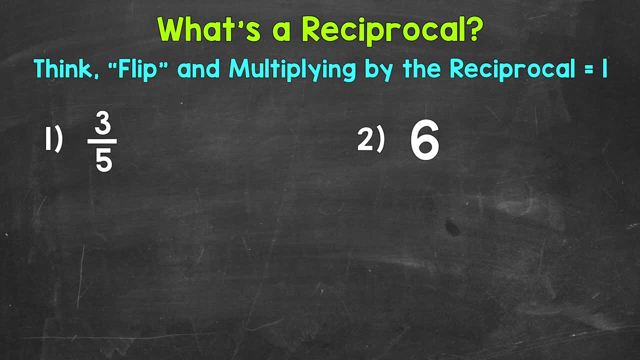 So let's find the reciprocal, and we do this by flipping the fraction. So the denominator the 5, is going to become the numerator And the numerator the 3, is going to become the denominator. So we are flipping the fraction. 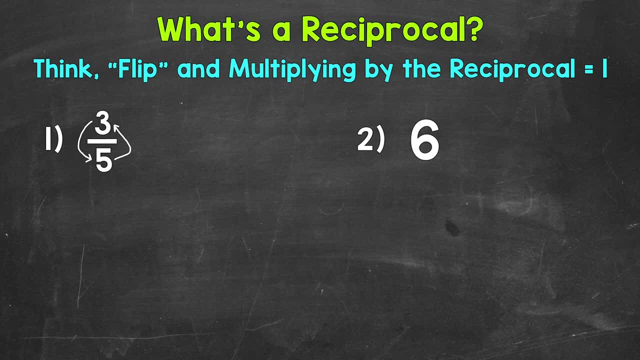 The reciprocal of 3 fifths is 5. 5 thirds. So that's our reciprocal. Now let's multiply our fraction 3 fifths by the reciprocal 5 thirds to show that we get 1 when we multiply by a reciprocal. 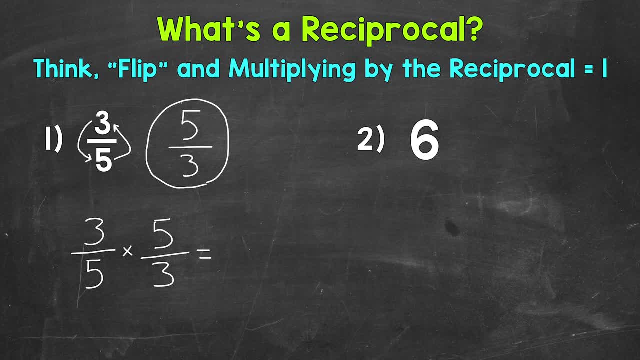 So let's multiply straight across The numerators 3 times 5, 15.. The denominators 5 times 3. Is 15.. So we get 15 over 15,, which we know is 1.. Whenever you have the same numerator and denominator, that fraction equals 1.. 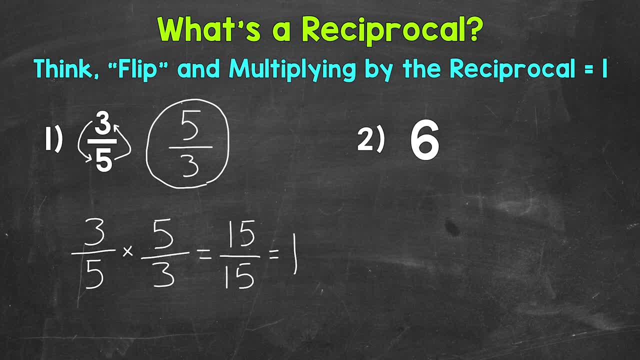 Let's move on to number 2, where we have 6.. For this one we have a whole number, So the first thing that we need to do is write this whole number in fractional form. That way we have a numerator and a denominator and we're able to flip that fraction. 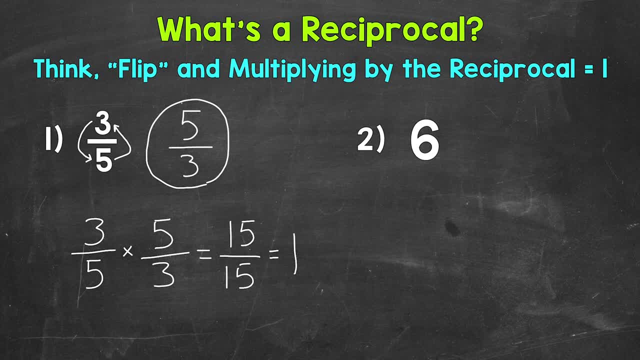 So to write a whole number in fractional form, all we need to do. I'll rewrite it underneath here. we put that whole number over 1. So that's 6 in fractional form. Now we're able to flip. So our denominator becomes our numerator and our numerator becomes our denominator. 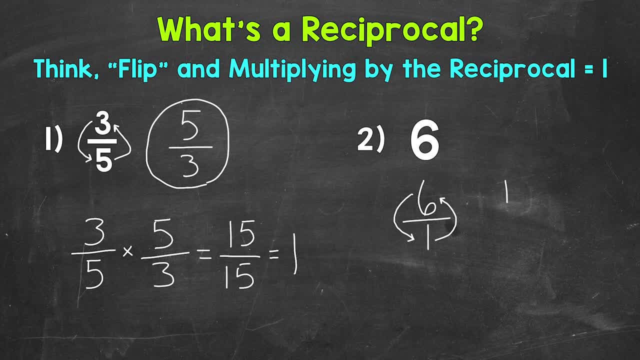 So the reciprocal of 6 is 1 sixth. This is our reciprocal. So let's multiply our whole number in fractional form, 6 over 1, times 1, sixth, to show that we get 1.. So numerators, 6 times 1 is 6.. 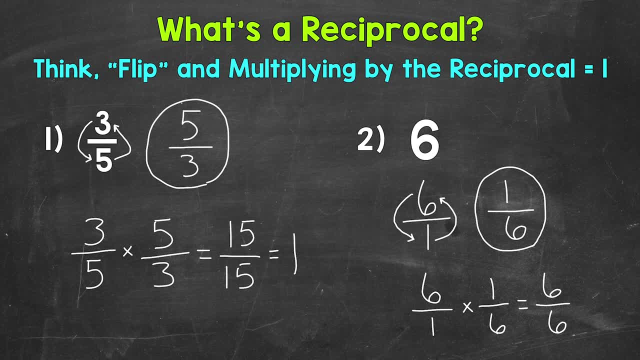 Denominators: 1 times 6 is 6.. Same numerator, same denominator: we get 1.. So again, when it comes to reciprocals, we need to think flip, And when we multiply by the reciprocal, we get 1.. 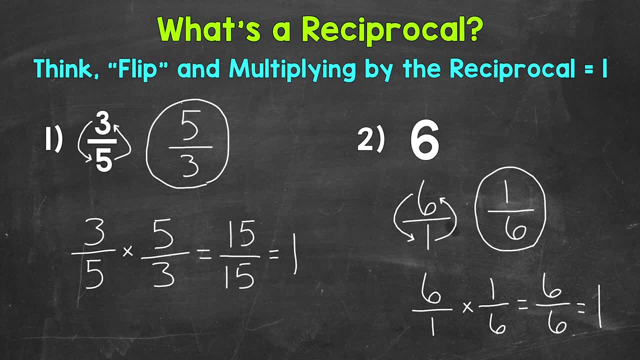 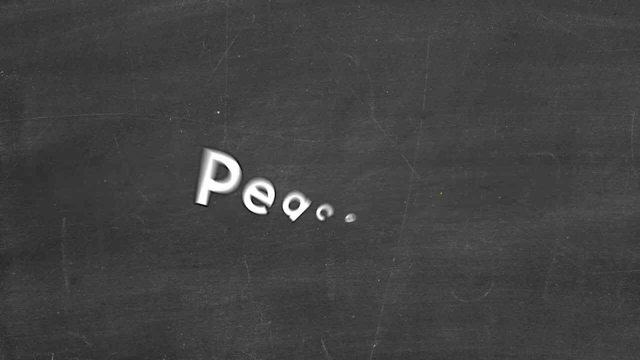 So there you have it. That was a basic explanation of reciprocals. I hope that helped. Thanks so much for watching. Until next time, peace. 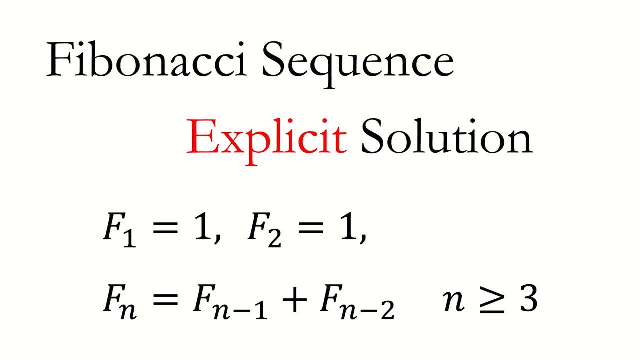 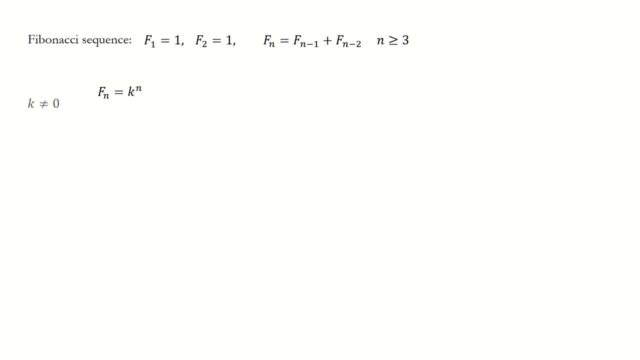 Hello, today let's derive the solution formula for the Fibonacci sequence And we will use this formula in the next video. So let's get started. First, we define the solution ansets into this form: And k is non-zero, So we got fn-1 and fn-2.. 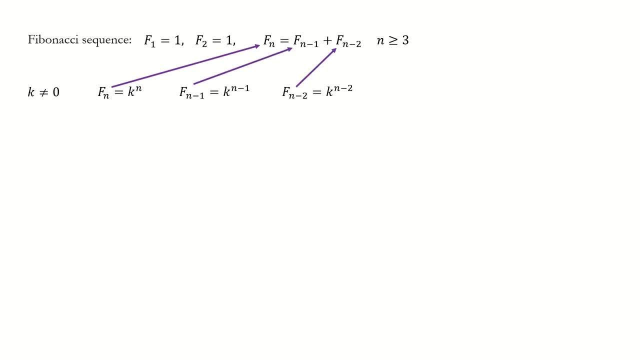 Next we plug them into the recurrence equation. And we got here. Then we divide this green term on both sides After canceling out the power index. we got this quadratic equation, Solve it and we get this, And we got two roots. 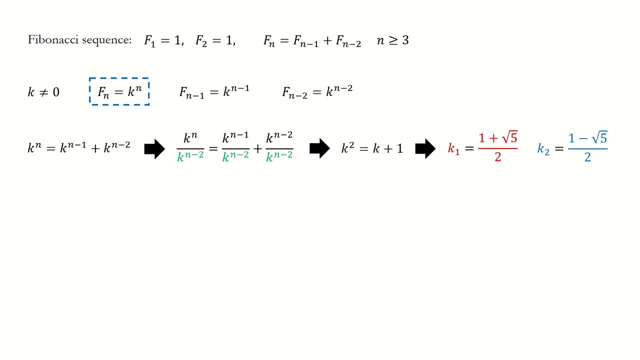 Since we define this solution into this form, we replace k by k1 and k2.. So we got two linearly independent solutions. The general solution can be written as the linear combination of these two solutions. Next we need to calculate the coefficients for c1 and c2.. 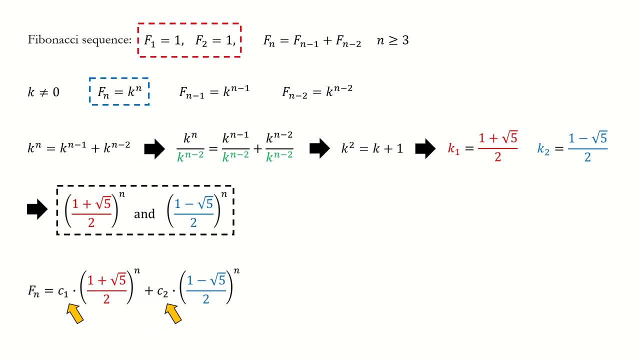 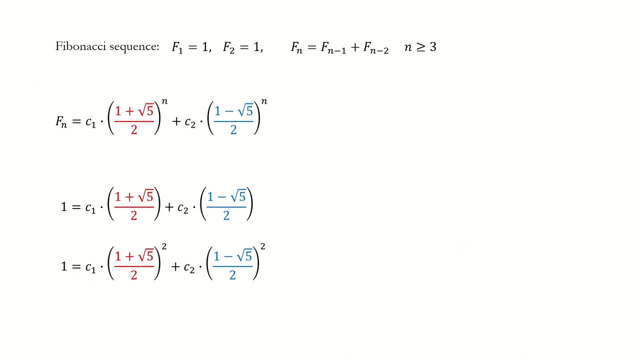 Then we are done. Now we use the initial conditions. So we got two linear equations for c1 and c2.. I copy them here. From these two equations we can solve for c1 and c2.. Plug in them and we got the final answer.